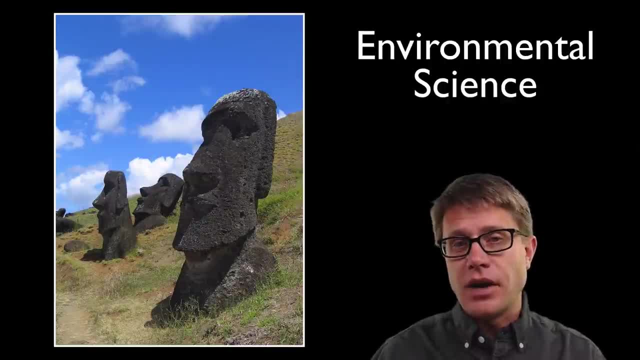 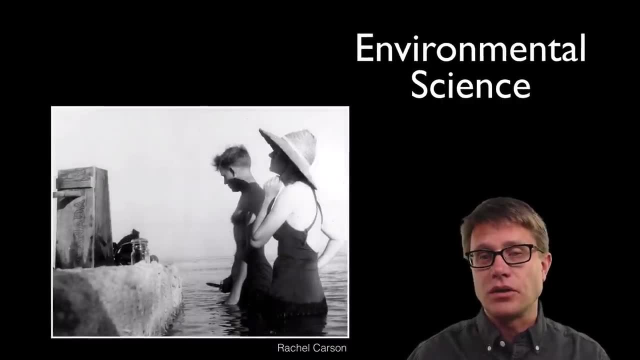 the island itself And their population dropped off dramatically, And so, as we study environmental science, we will deal with very important figures, But I wanted to begin with a very important figure named Rachel Carson, And she really brought us into the modern age of environmental 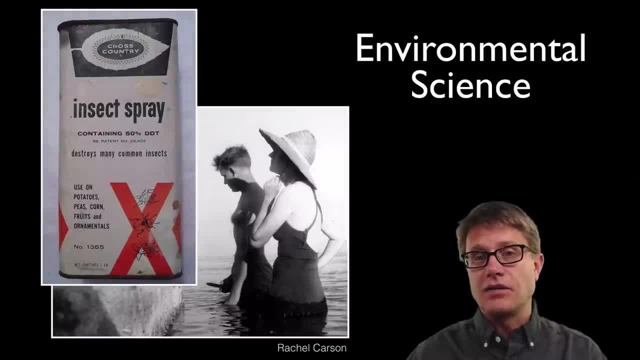 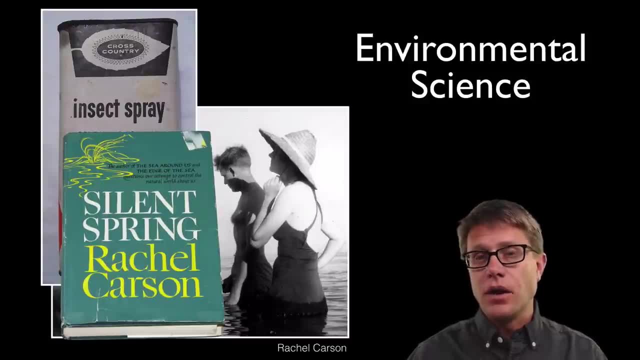 science. Her study of DDT and the negative consequences of that, which are illustrated in her book Silent Spring, really brought that to the forefront of our minds. What are we doing And how are we impacting the environment itself? And so this is an environmental science. 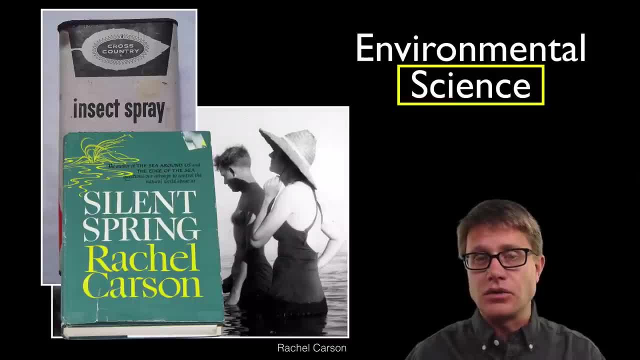 And so, like any other science course, we are going to deal with a scientific method. Now, sometimes students will confuse that term with environmentalism. Now, that is going to be a belief system, So we are going to lobby officials and try to get laws passed that 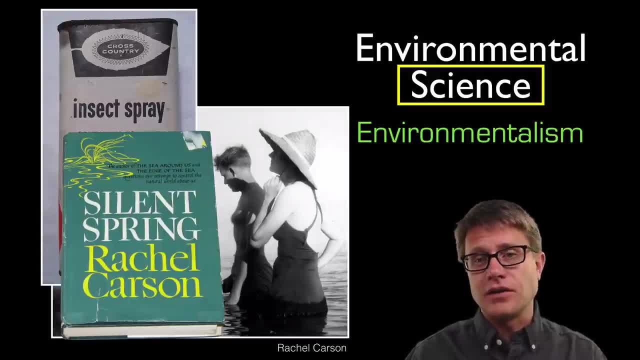 protect the environment. That is not environmental science. Environmental science is looking for that truth of how we can interact with the environment. So maybe in the future science will say that DDT is an important tool that we could use to fight malaria, And that is. 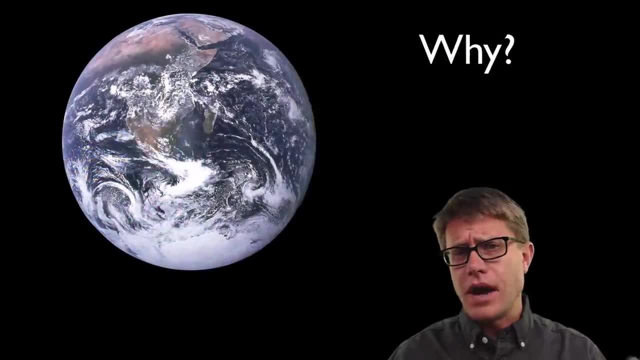 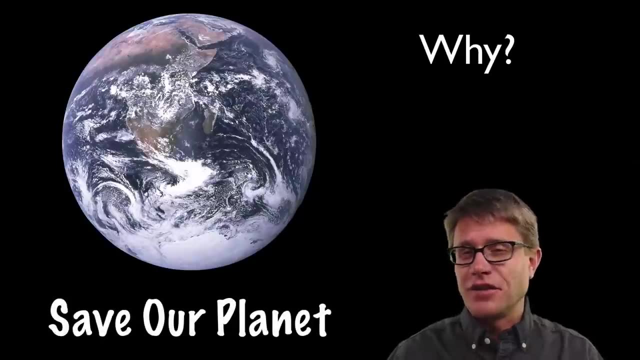 true, Then we have to follow that pathway. And so why is this course important? Well, when I was young, people used to wear t-shirts that said save our planet, And it is kind of a funny shirt, Because the planet, the earth, is going to do fine. It is how we do. 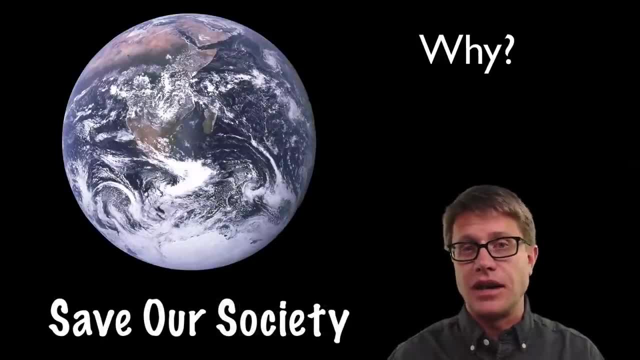 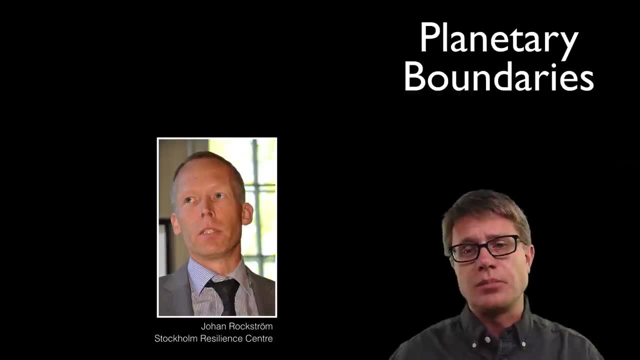 on that planet that is important to us, And so a better slogan is: save our society. And why is that a big deal right now? Well, we are studying to exceed some what have been coined planetary boundaries by Johan Rockström, And Johan Rockström is one of the most famous. 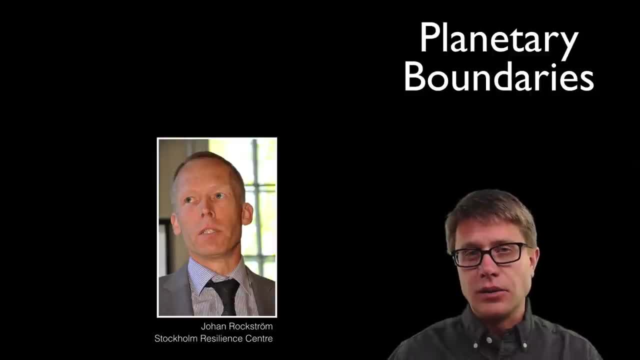 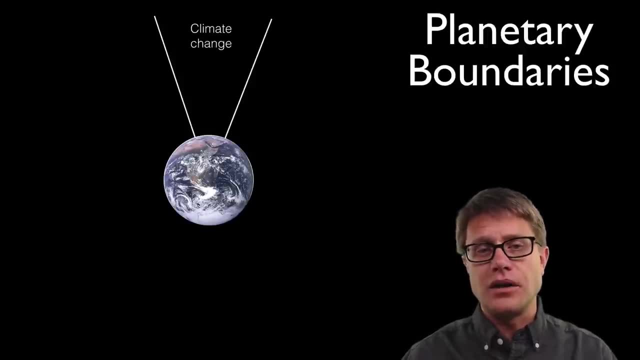 scientists in the world, And he and his group at the Stockholm Resilience Center, And so if we look at this model, we look at all the things that are affecting the earth that can then affect society, And so the one that you are probably familiar with is climate change. 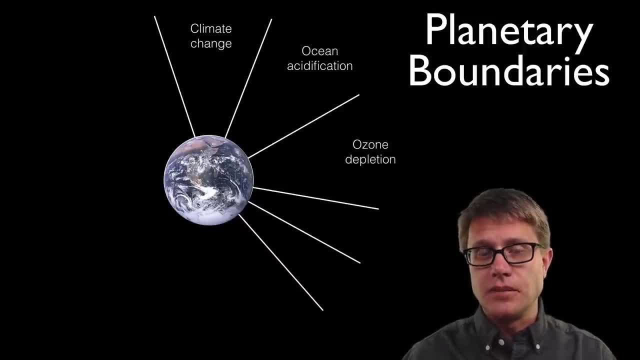 But we also have ocean acidification, We have ozone depletion, We have changes in biogeochemical cycling, Increases in nitrogen and phosphorus. We have fresh water use or the availability of fresh water, Deforestation, Biodiversity loss, Particle pollution and chemical pollution. 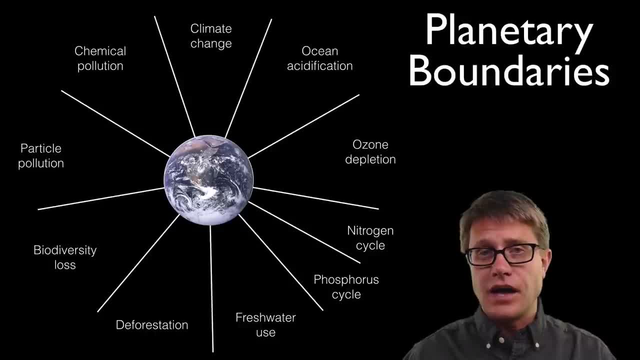 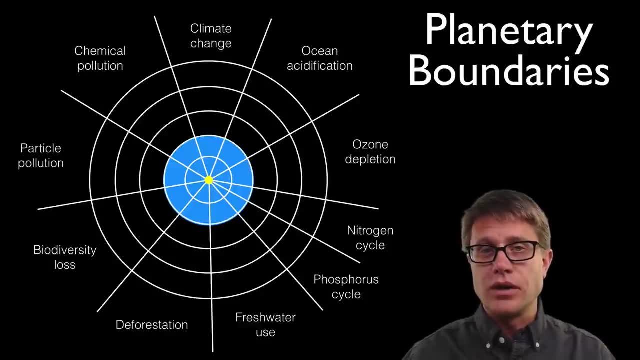 So we have all these things that are affecting the earth, And so we have changes in biogeochemical pollution, And so what they have done is said: how can we exist within the safe boundaries of the earth? So, on this model, if we say the blue represents where we can safely live. 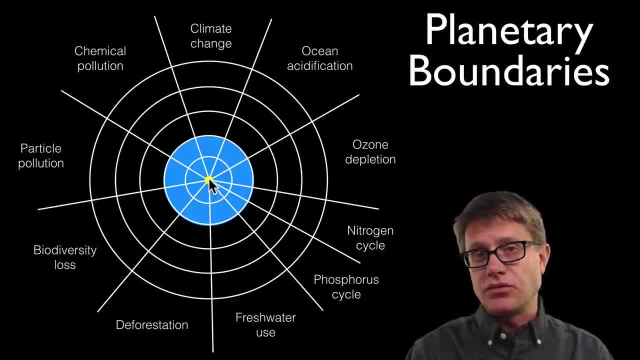 this yellow dot represents where humanity was: pre-industrialization, Before the industrial revolution and the spread of industry around the world. these were our levels, But now, if we look at where we are as far as those boundaries, as far as climate change, we are. 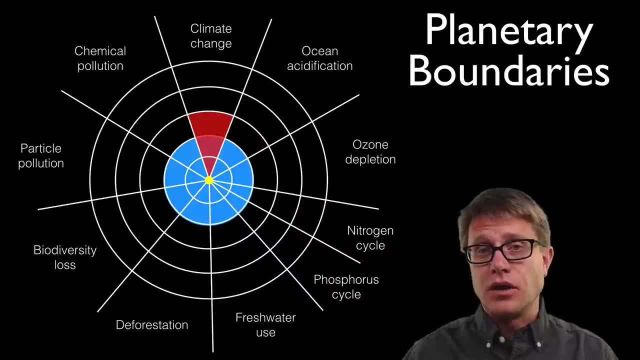 increasing the climate, the temperature And, as a result, we are going to have consequences that are beginning to affect society and will continue to affect society. We are looking at a 3 degree increase, which is incredible, But if we look at these other ones- ocean. 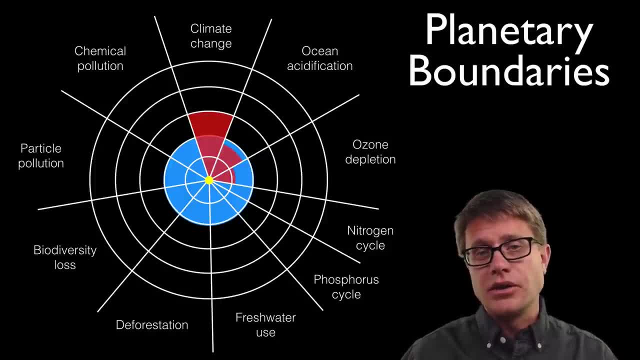 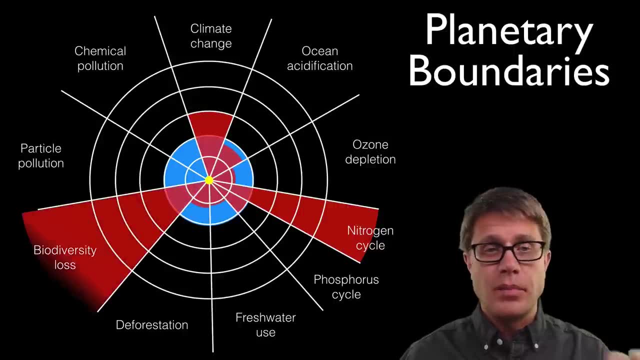 acidification, ozone depletion, our increase in the amount of nitrogen in the biosphere, phosphorus. If we look at fresh water use, deforestation, biodiversity loss. a lot of scientists say we are headed into the sixth extinction And so we are going to have a. 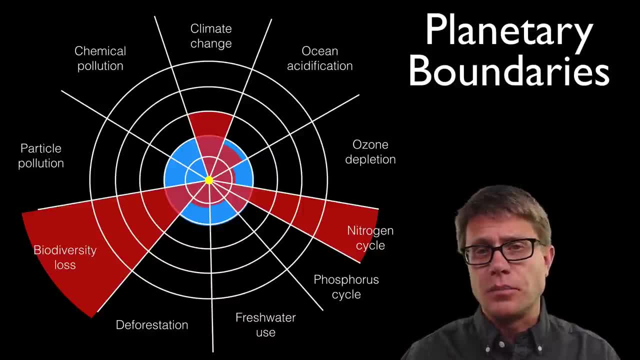 second extinction caused by humans. Now we do not have good models for pollution. but if you put our earth back, we are exceeding these boundaries. We are putting pressure on the earth Now. the earth will survive, but humans may not survive in the numbers. 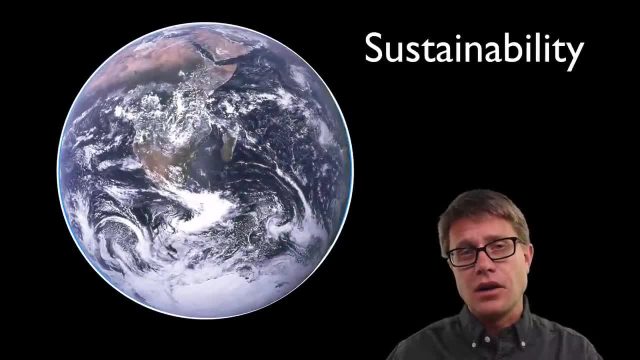 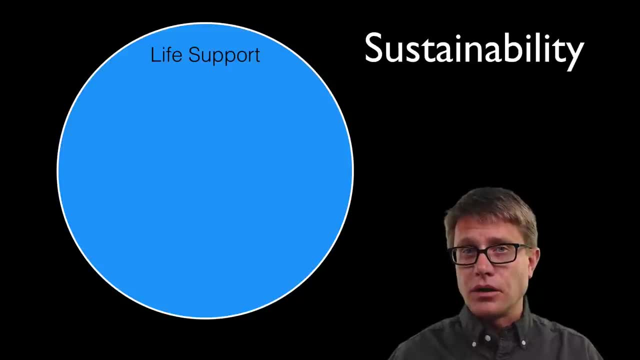 that we are today, And so that is why it is important We have to live within the boundaries of the earth itself, And so sustainability is incredibly important. Now, a model that works is since industry brought us to this point. industry is going to have to bring 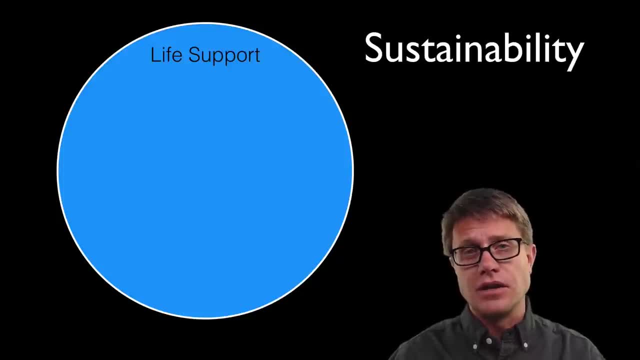 us back. model works for me. If you think of the earth as this boundary of life, support, and society exists within that, then what is at the center? What drove industrialization? It is the economy, And so, as we come up with solutions for sustainability, it is not enough to just say that we should. 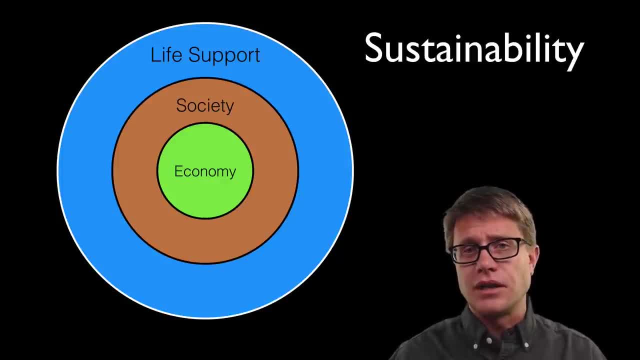 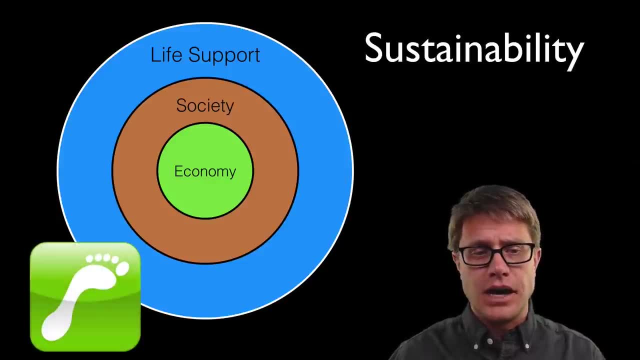 save the earth because that is good, Or we should be altruistic in that It has to be an economical driver that is pushing that sustainability. Another term that you will hear a lot is the idea of an ecological footprint, Since we- I live in a developed country. I 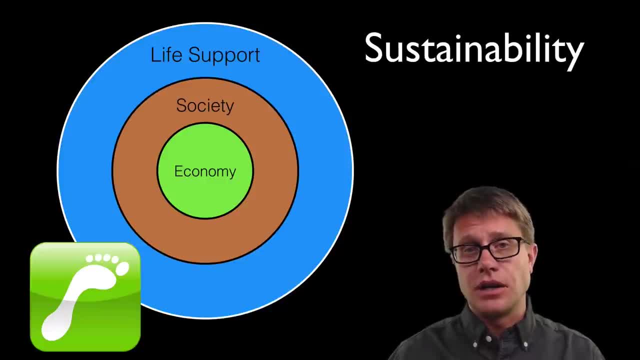 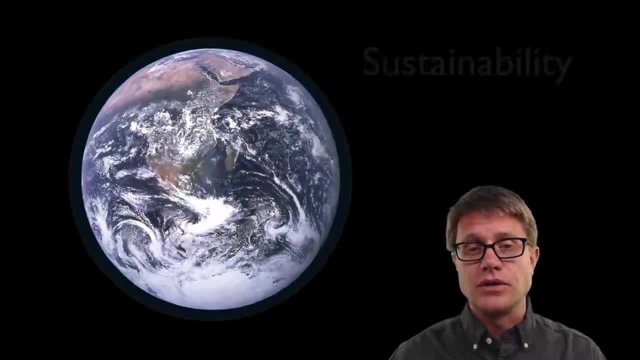 am using more resources on our planet than other people in developing countries, And so, as they become developed, that is going to put even more pressure on the planet, And so that is why this course is incredibly important. It is also why this is unlike the other sciences. 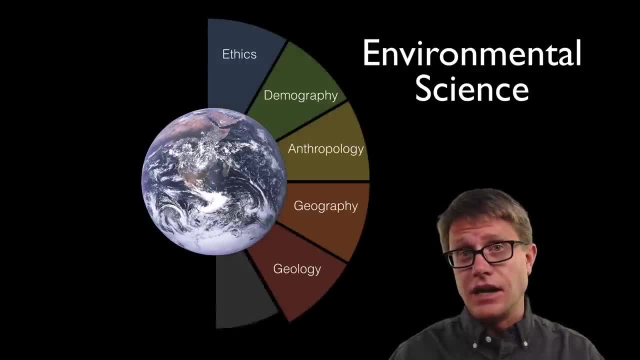 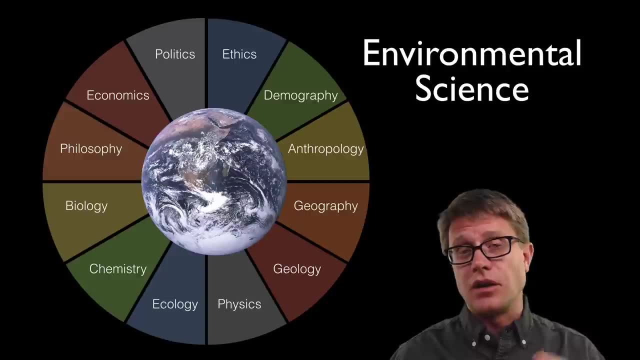 that you have probably taken. It is not just going to be science. It is going to contain the natural sciences, But it will also have the social sciences and the humanities as well. So we are going to be talking about science, But also we will be talking about ethics and 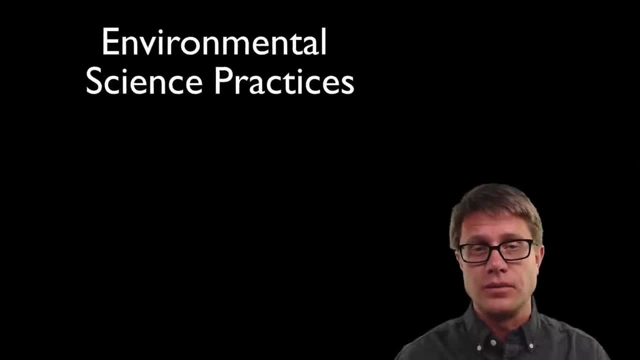 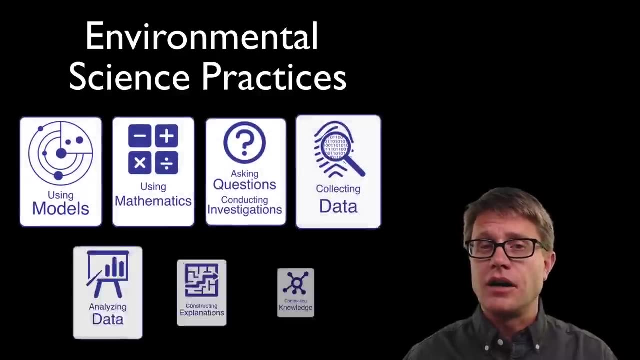 law and politics, And so it is really going to be a fun course to walk through. Also, you should remember that this is a science course, And so, as we move forward, the AP folks are focusing on the practices of science. So inside the course itself, you should be acting like. 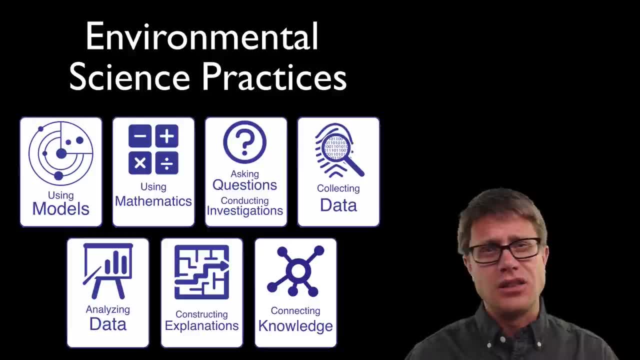 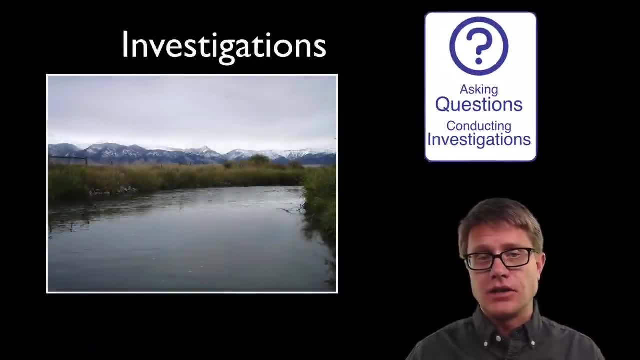 an environmental science scientist, rather, And so you should not just be learning about environmental sciences, You should be applying it. So if we start with one of these practices- asking questions, conducting investigations- this would be a great field investigation for me to do. So this is the Eastern Gallatin. 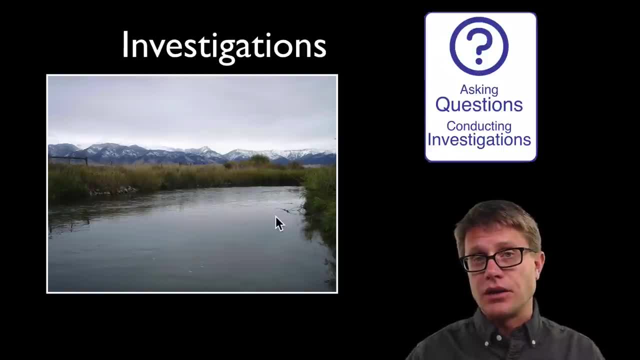 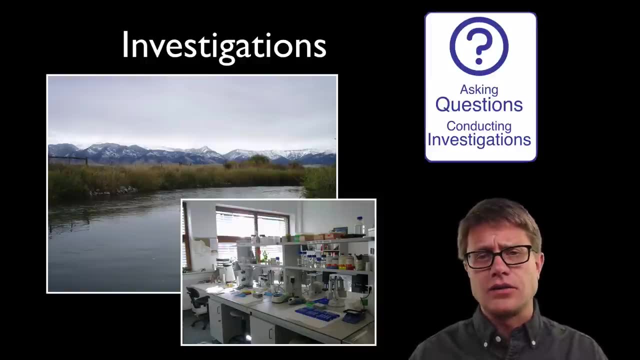 right outside Bozeman And so I could do studies here on water quality over time. But I could also do studies in the laboratory. I should be doing investigations where I am coming up with a question and trying to answer that question. Case studies will be incredibly. 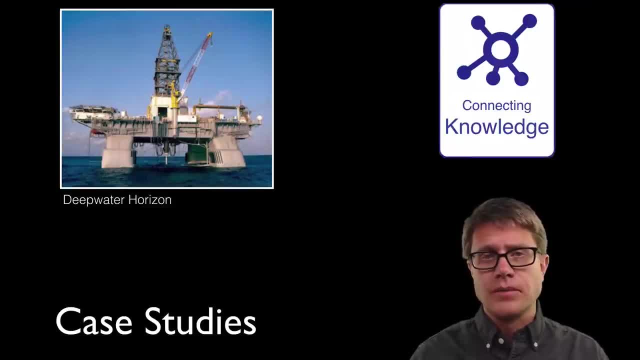 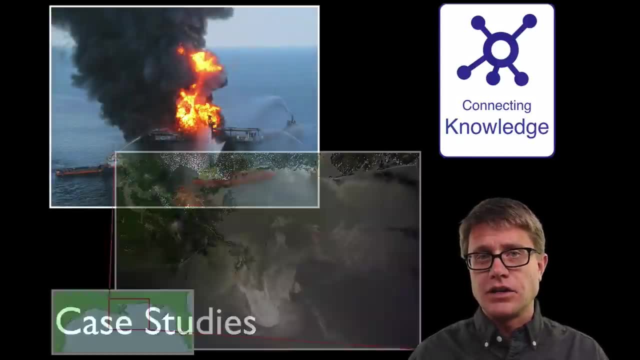 important as well: Making these connections between what we have learned in the course. So you are probably familiar with the deep water horizon. There was a fire and that led to this spread of oil. So this fire. eventually there was a breach of the pipeline And so 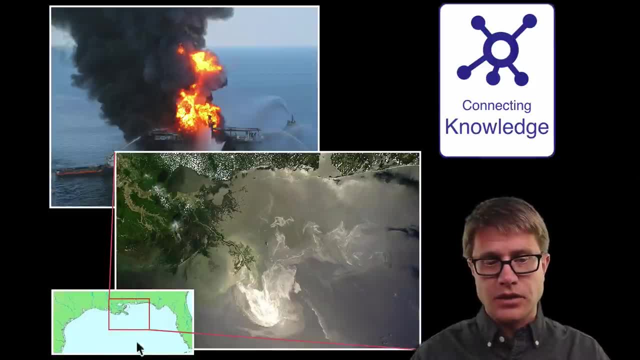 we have a pipe and now we have oil spreading. So, to look at where we are, this is in the Gulf of Mexico, This is Florida, And so we are looking at this area right here. You can see so much oil is spread out And in each of these case studies there is something happening. 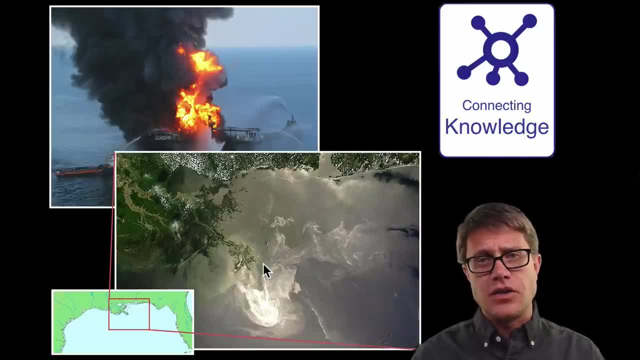 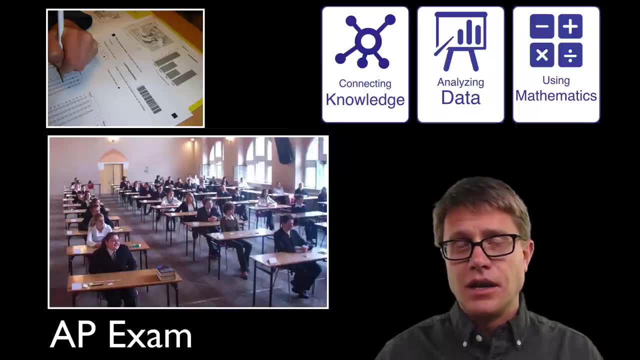 to the environment, And so we have to understand all the ramifications of that, And lots of times it takes decades to figure out what really has happened, And then, finally, you are going to take an AP exam at the end, And so understanding how that AP exam is important, 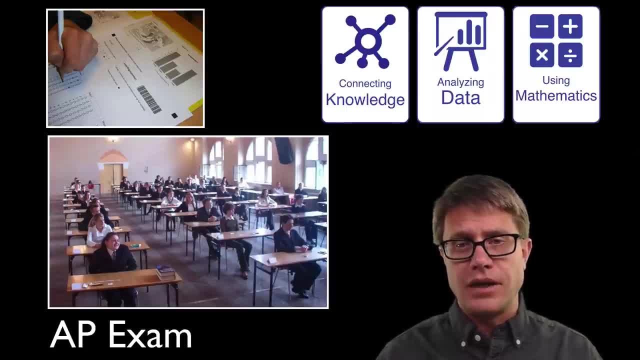 right now to understand what can you do throughout the course to kind of prepare for that And so, and then you are going to take an AP exam at the end, And so understanding how that works, analyzing data using mathematics, is going to be incredibly important, So let